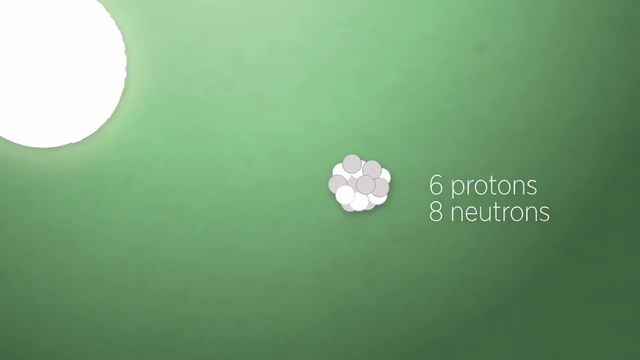 and protons off of others And, before you know it, the nice, stable family man nitrogen-14 atom is all wrapped up and gone crazy and becomes what's known as a carbon-14 atom, which is radioactive. Now carbon-14 atoms aren't the only ones in the upper atmosphere. 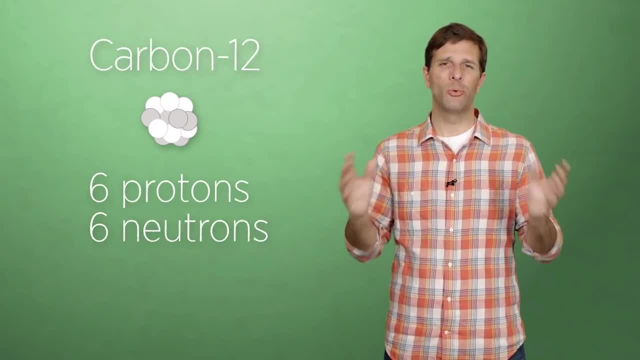 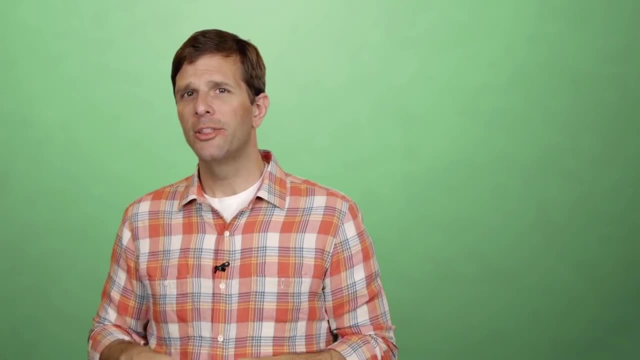 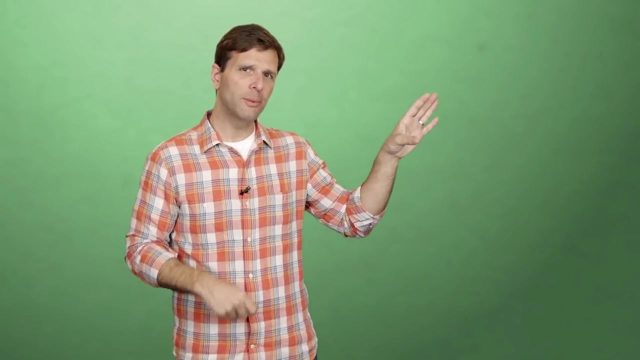 There's also carbon-12 atoms. Carbon-12 atoms are in much more abundance and they're pretty stable. Carbon-14 atoms are again radioactive and unstable, But they're formed at a reliable, steady rate. So at any point in time we have a pretty good idea of the ratio of carbon-12 atoms. 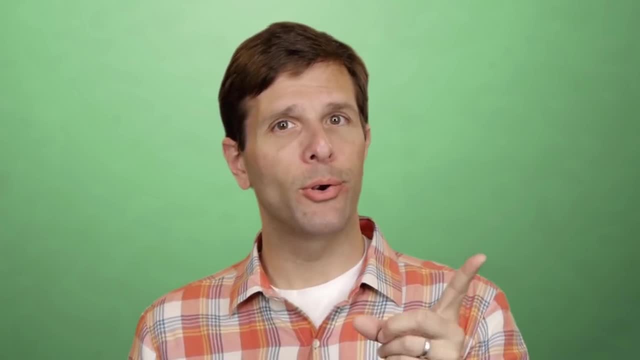 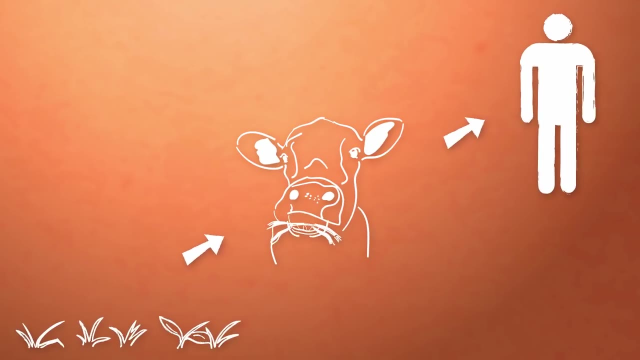 to carbon-14 atoms. Got that? It's important Now. carbon dioxide is essential to life here on Earth. Plants breathe it in, Animals eat the plants, We eat the animals and the plants, And these carbon molecules are the ones that are responsible for life on Earth, And they're 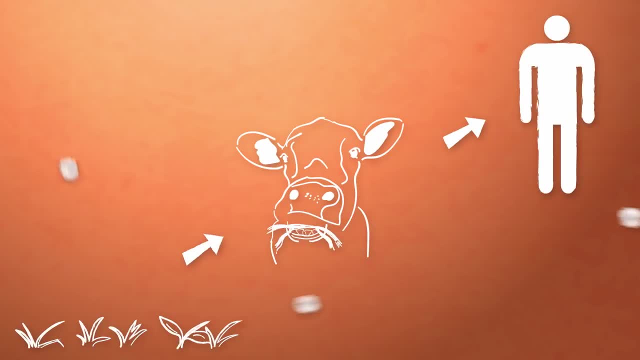 the ones that are responsible for life on Earth, And they're the ones that are responsible for life on Earth, And they're the ones that are responsible for life on Earth. And these carbon molecules- carbon-14 and 12, that make up the carbon, dioxide, get in everything. 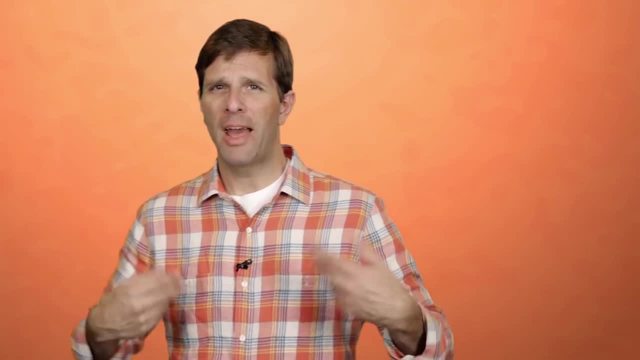 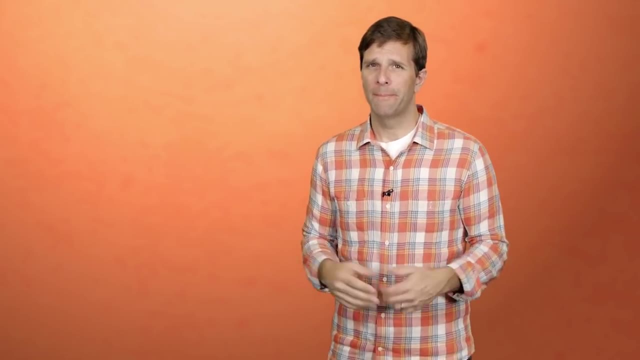 What's neat is that the ratio of carbon-12 to carbon-14, found in all these living things here on Earth is pretty much the same as what's in the atmosphere, which means it's predictable, And some very, very smart scientists have figured out that carbon-14 actually decays. 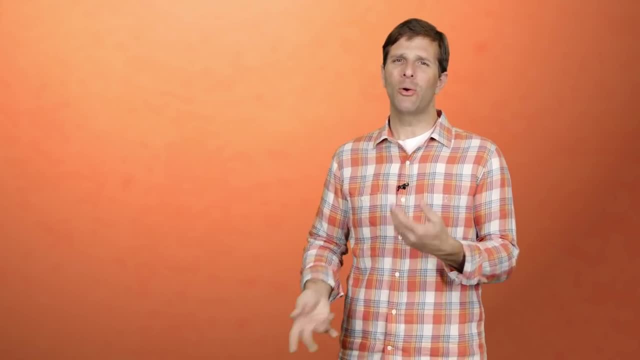 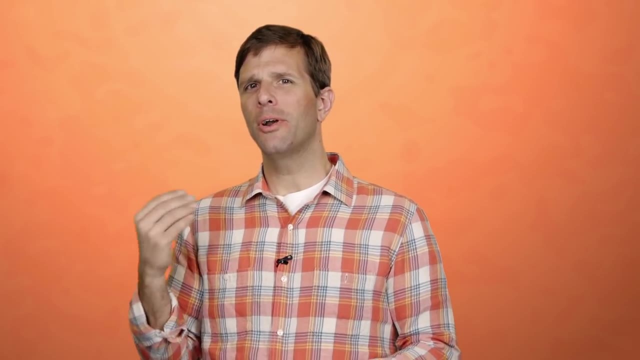 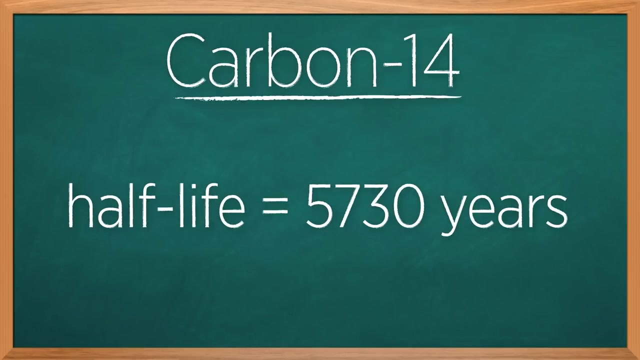 at a predictable rate right? Carbon-14,, like all radioactive particles, has what's called a half-life. A half-life is the amount of time it takes for the number of radioactive particles in a sample to decrease by half. Carbon-14 has a half-life of 5,730 years. That means that 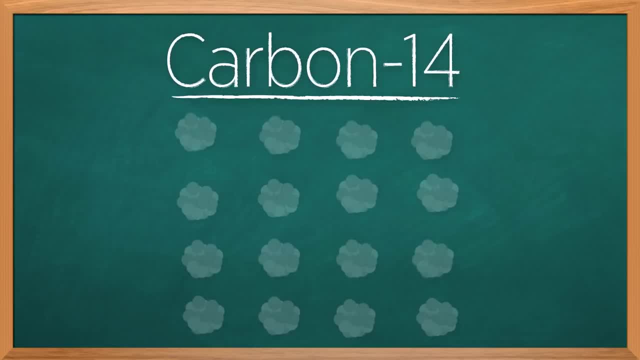 after 5,730 years, the amount of carbon-14 atoms in a, say, plant that you found fossilized will be half of what it was the last time that plant took well, a breath of life. After 11,460 years, which is two half-lives, there'll be a quarter of that half-life And that's. the amount of time it takes for a plant to decrease by half. Carbon-14 has a half-life of 5,730 years. That means that after 5,730 years, the amount of carbon-14 atoms in a, say, plant that you found fossilized will be half of what it was the last time that plant took. well, a breath of life And that's the amount of carbon-14 atoms in, a, say, plant that you found fossilized will be half of what it was the last time that plant took, well, a breath of life. And then, after 17,190 years, you'll have just an eighth of the number of carbon-14, and so on and so 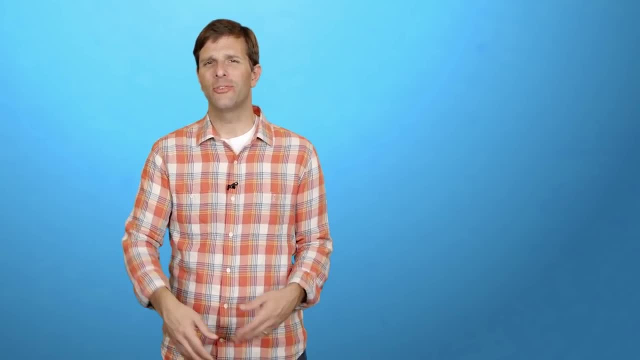 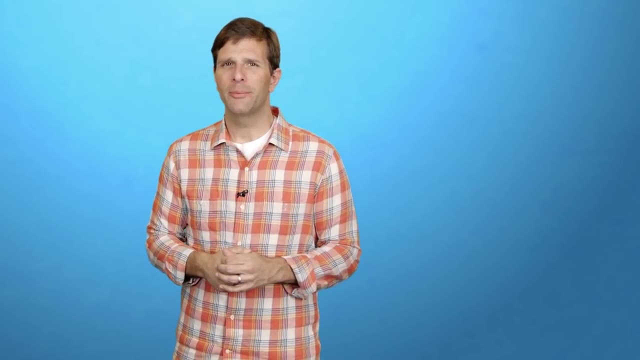 on until there's none left. And this is actually one of the limitations of carbon-14 dating: that eventually you're going to go far enough back in time that all of the carbon-14 atoms have decayed And you don't know whether this took place a day before or a hundred thousand.